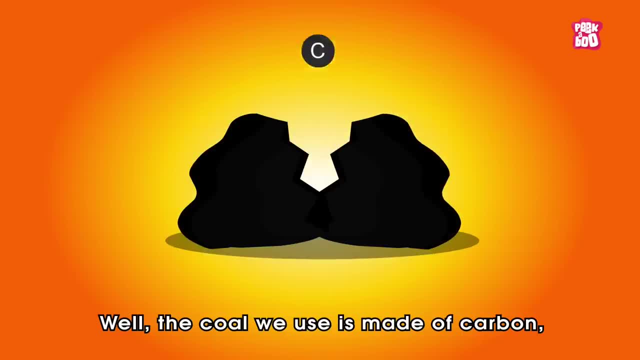 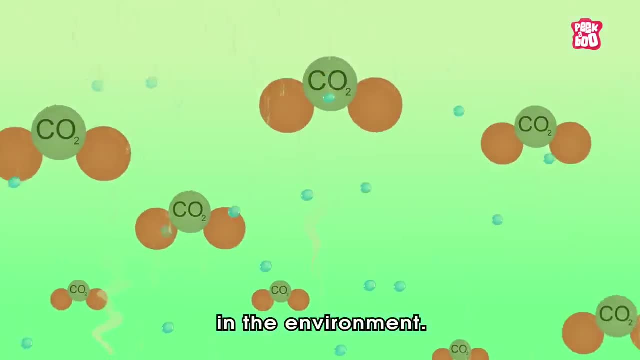 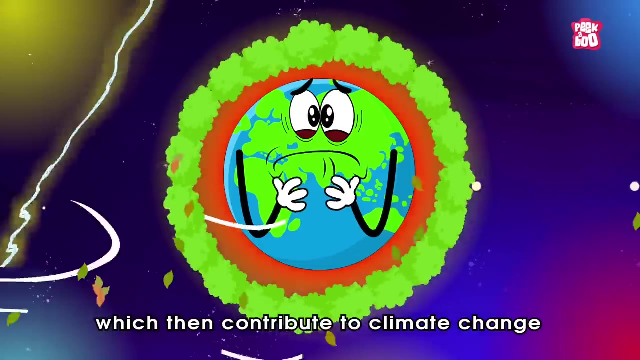 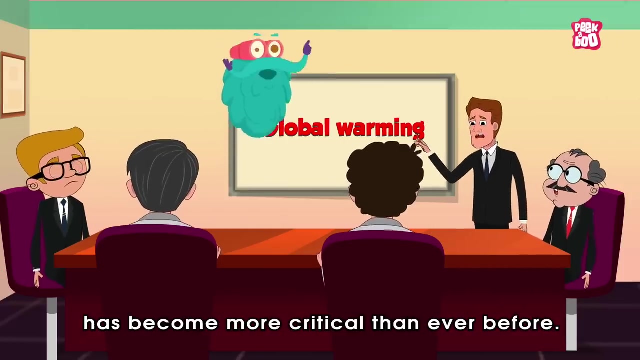 Well, the coal we use is made of carbon, And when mixed with oxygen, it leads to an increase in carbon dioxide. This eventually contributes to greenhouse effects, which then contribute to climate change and cause global warming. Hence, the need to find a suitable alternative has become more critical than ever before. 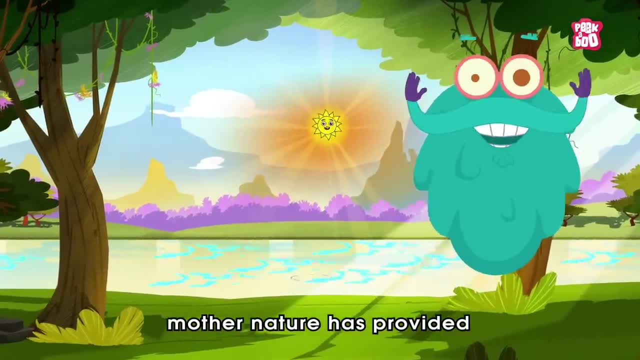 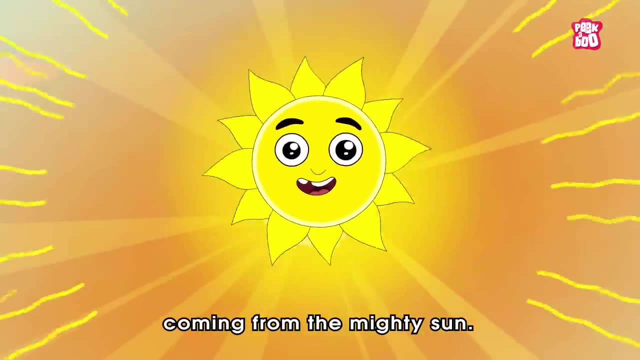 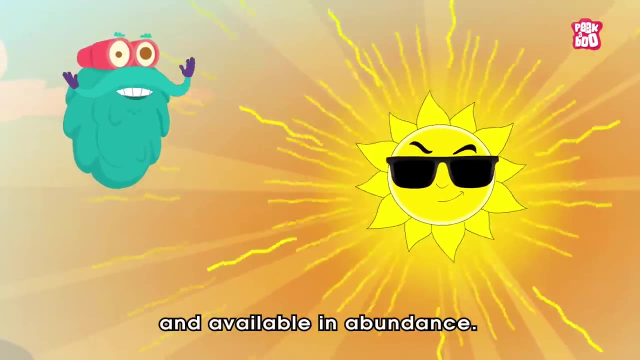 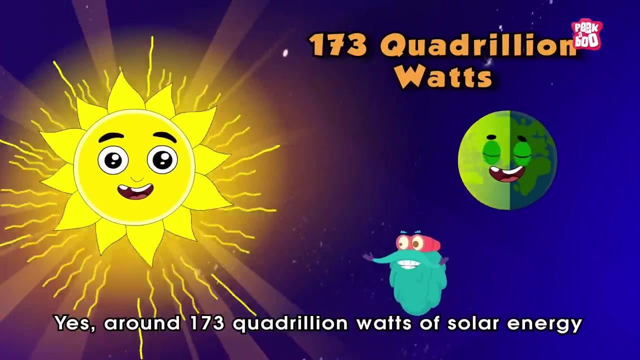 And fortunately, Mother Nature has provided an alternative solution in the form of solar power coming from the mighty sun, And the best part is it is absolutely clean, free and available in abundance. Yes, around 173 quadrillion watts of solar energy strike the Earth continuously. 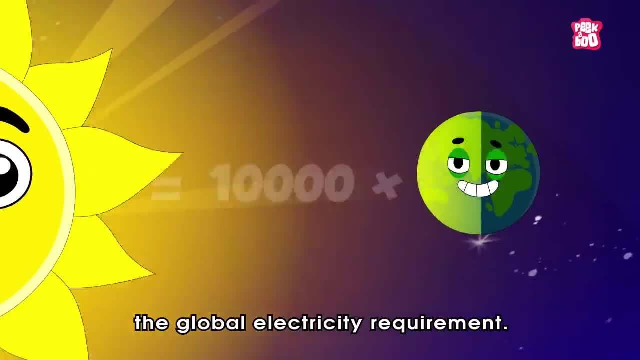 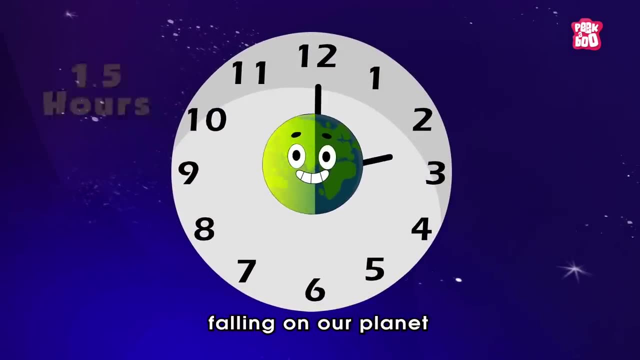 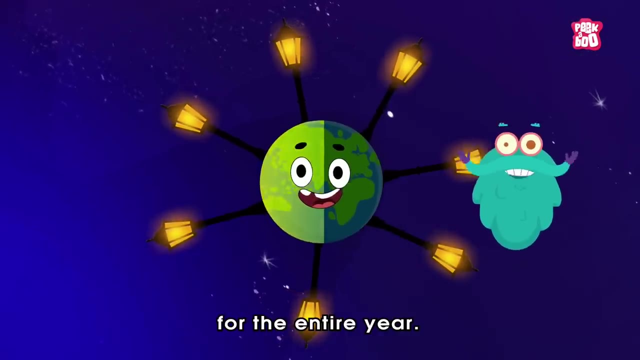 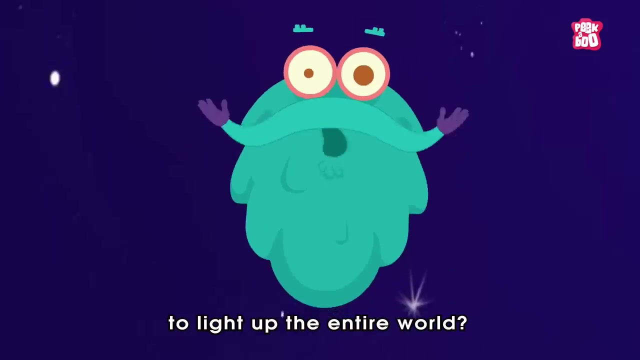 That is 10,000 times the global electricity requirement. So it means a mere 1.5 hours of sunlight falling on our planet Is enough to fulfill the world's energy consumption for the entire year. But the vital question is: how could we capture this solar power to light up the entire world? 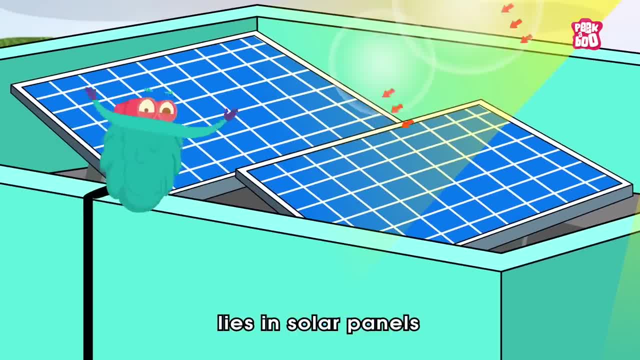 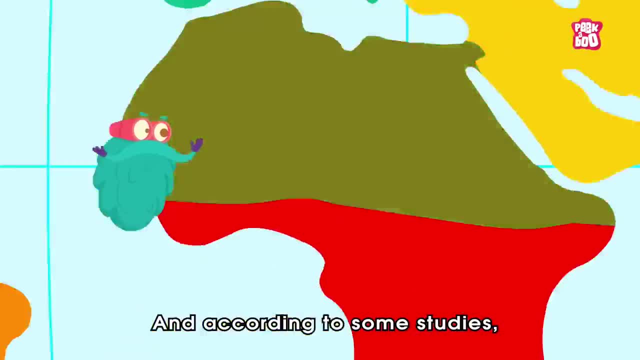 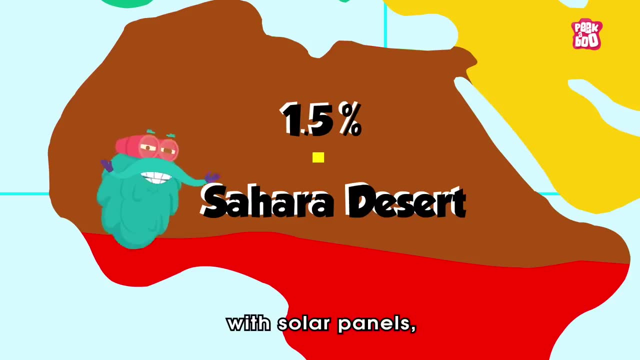 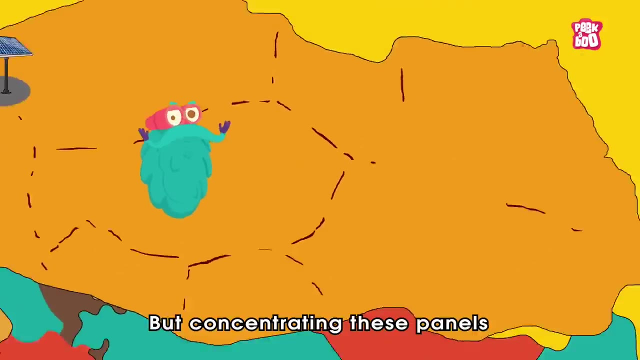 The answer to this question lies in solar panels that are used to convert sunlight into electricity, And, according to some studies, even if we cover 1.5% Sahara Desert with solar panels, there could be enough to meet the global electricity requirements. But concentrating these panels in one place would cause many hurdles. 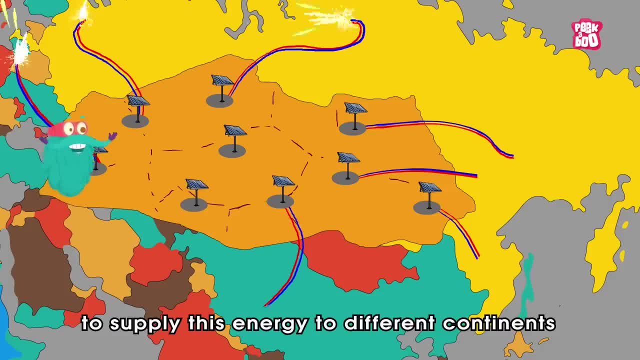 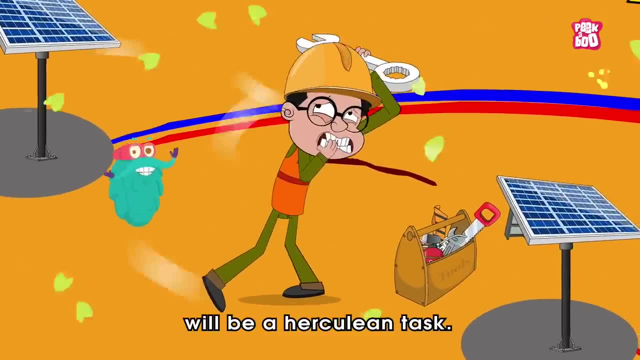 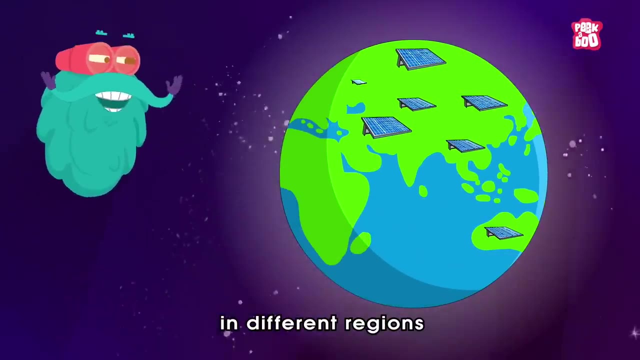 as it will become difficult to supply this energy to different continents, and even maintaining this facility will be a Herculean task. Therefore, a better option is to use solar panels. A better option will be to install these solar panels in different regions. where there is abundance of sunlight, like they did in Bhadla Solar Park, located in Rajasthan, India. This is the largest solar park in the world, which is spread around an area of 56 square kilometers, And all we need to do is build about 9,000 such facilities.